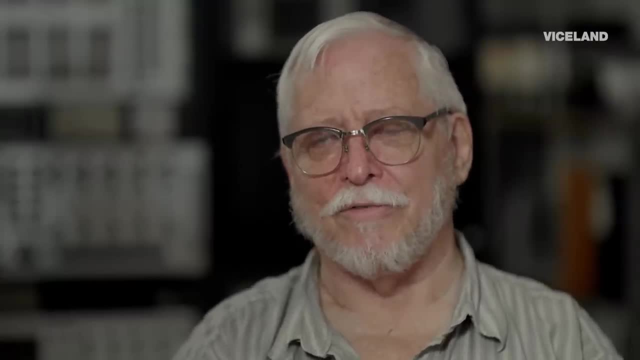 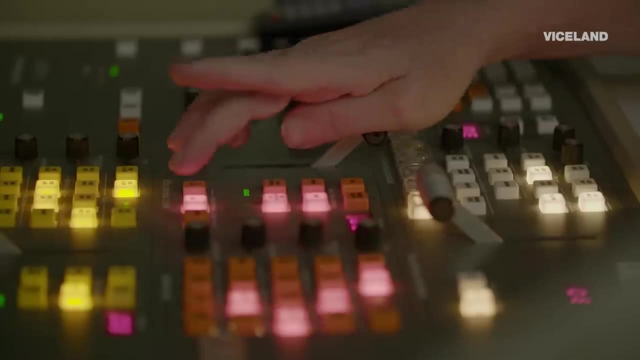 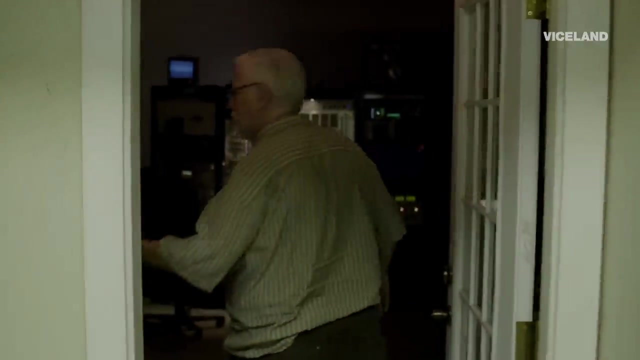 of one of the 10 Scanimate machines that was ever built. NBC Sports, ABC Sports, CBS Evening News. We had a scene in the first Star Wars. It was everywhere. This is the Scanimate room. It's gotten hot in here. 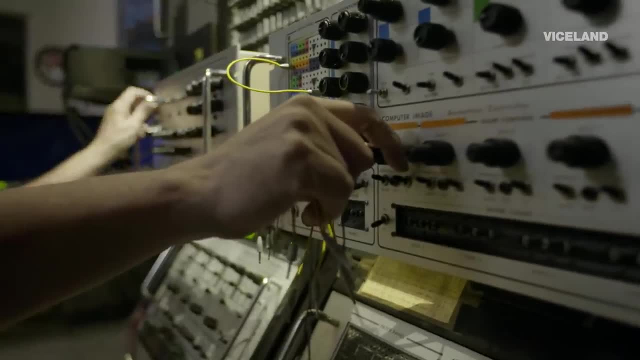 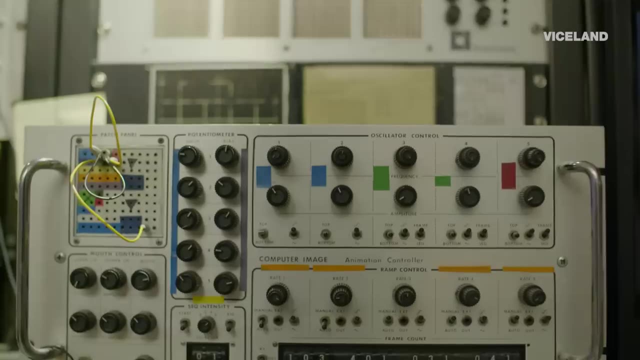 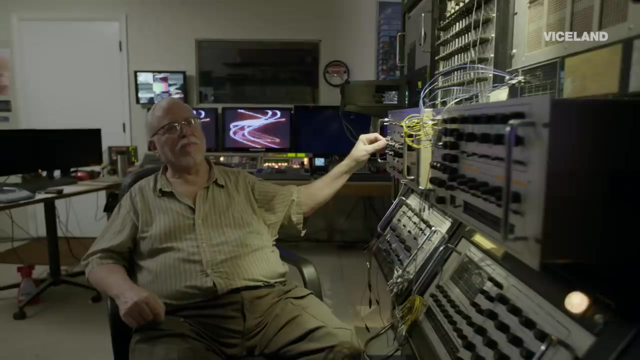 These are the only two that I know of that work. I have the first R&D machine and I have the last one ever produced. It's just got a very distinct look that can't be replicated. It's sort of the visual equivalent of like a Moog synthesizer. 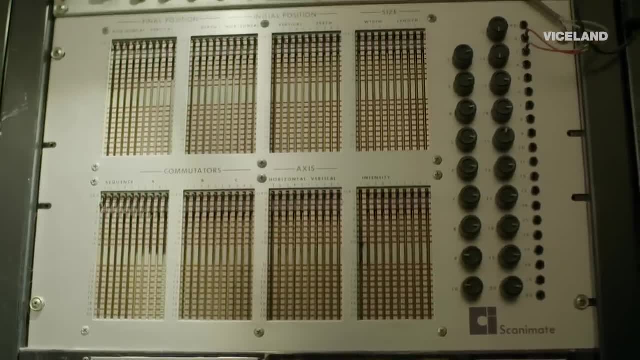 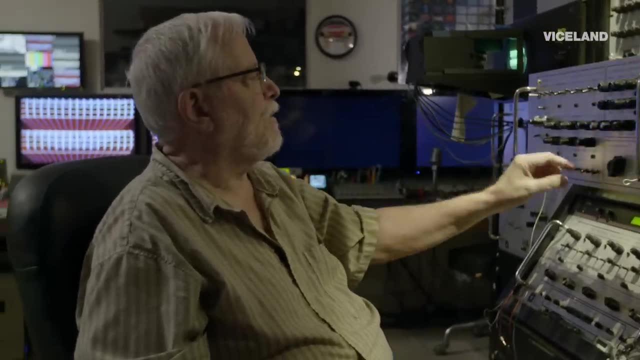 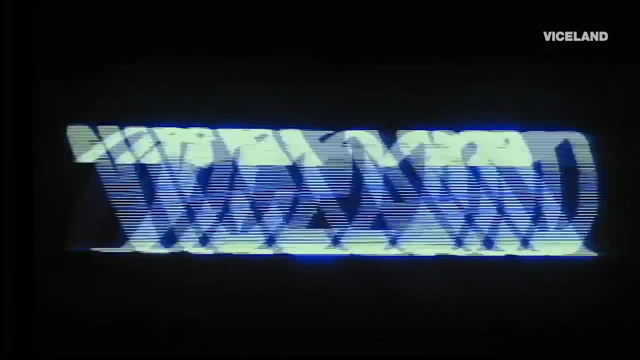 With analog, it's a continuously variable thing that you can adjust When it's in the initial position. I'm going to put an oscillator. I'm going to put an oscillator on depth. One of the nice things about the Scanimate is that as you adjust something, as you turn. 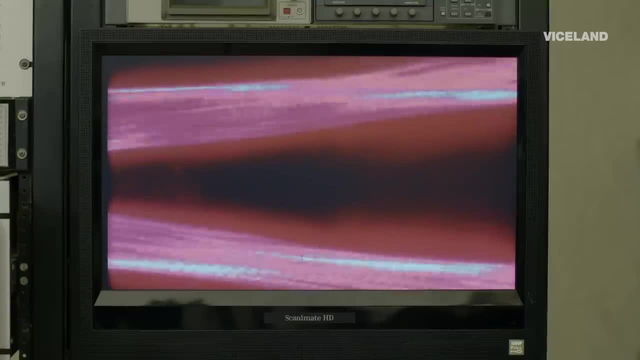 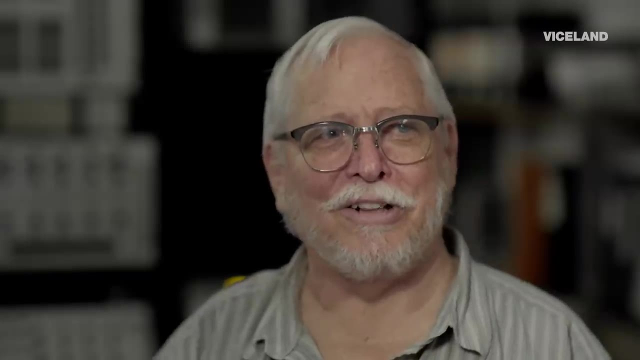 the knob. you immediately see it. It's just continuous. That's analog. You plug in things to make your animation. I mean, that's really where the term plug-in came from. It's very tangible. You can affect the image with your hands. 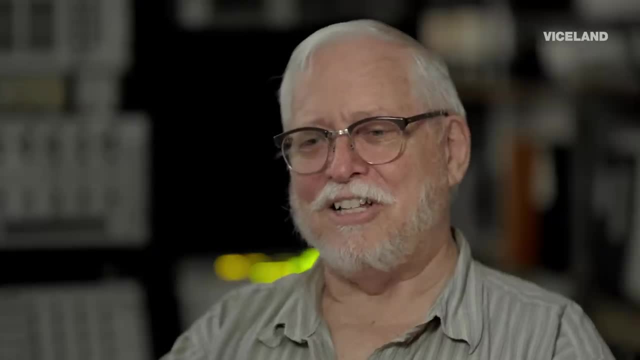 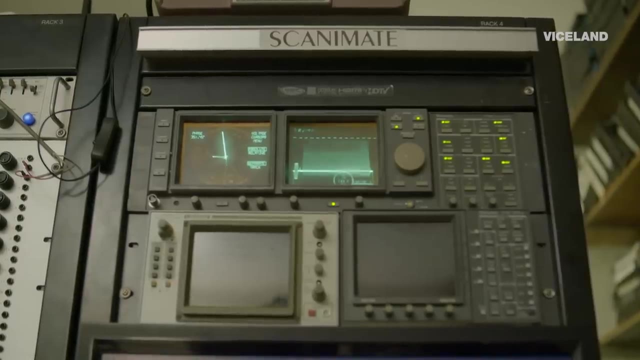 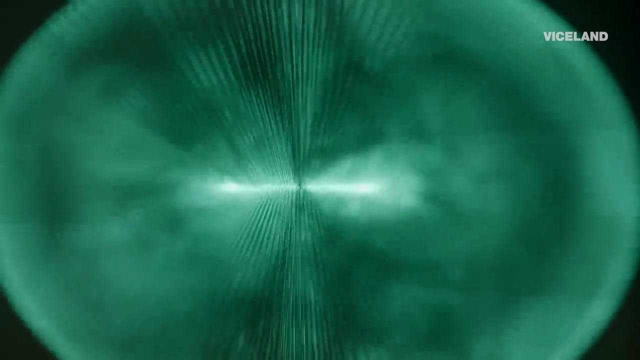 I mean, you can almost touch it. You can't touch any of this digital stuff. It's in the computer somewhere With the Scanimate. you're literally photographing light that's coming off a phosphor screen. This is a very abbreviated version of the animator's cheat book. 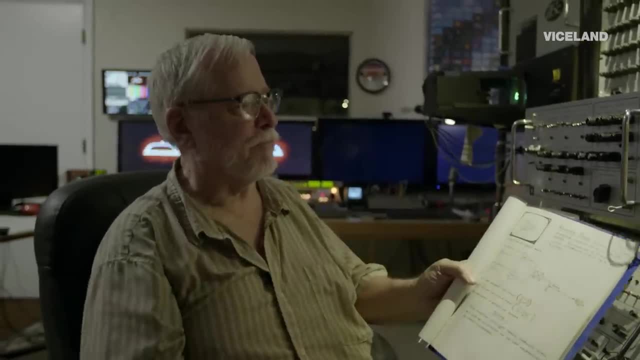 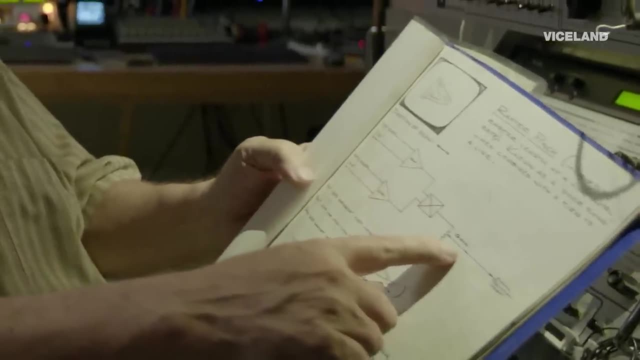 For example, if you've got a logo and you want it pushed back in perspective, you can do that. You have a horizontal ramp to a semi-amp with a bias pot. multiply them together into a gain pot and feed that to final section, vertical.